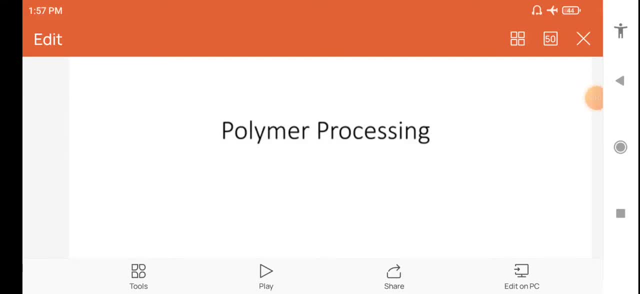 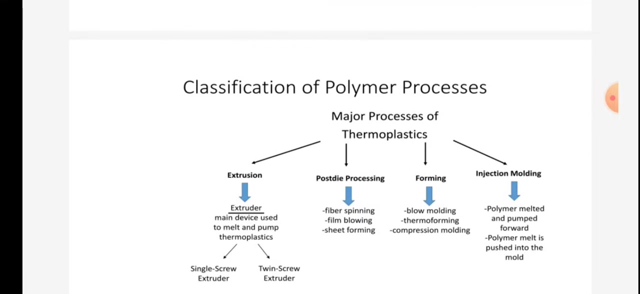 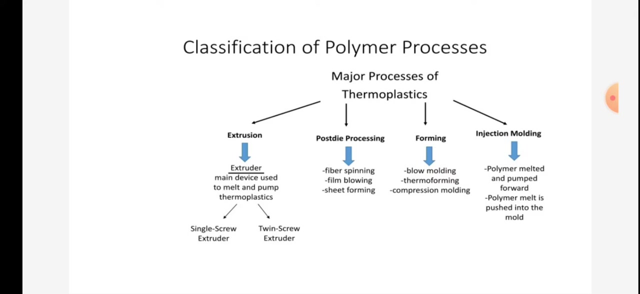 Welcome back, friends. We are seeing the subject: manufacturing process In this process, the unit of polymer processing we are now studying In this process: polymer processing. classification of polymer processes. Major processes of thermoplastics are as given below: Extrusion, post die processing, forming and injection molding. These are the subtopics of major processes. polymer processes. Extrusion: In extrusion, extruder is given main device used to melt and pump thermoplastics. In this there are two topics. 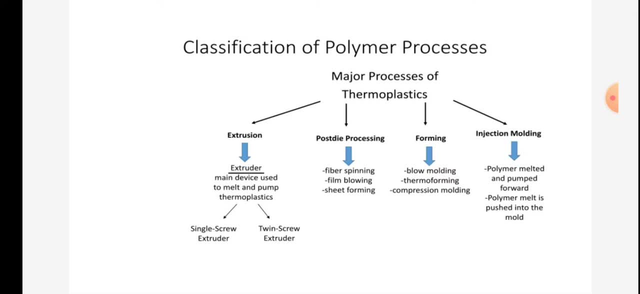 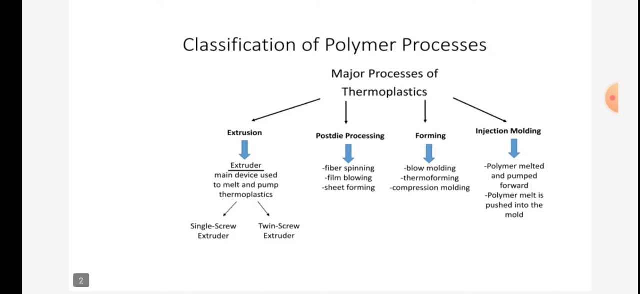 Single screw extruder and twin screw extruder. Post die processing In this process: fiber spinning, film blowing, sheet forming. Then forming In this forming process: blow molding, thermo forming, compression molding, Injection molding is given by polymer melted and pumped thermoplastics. 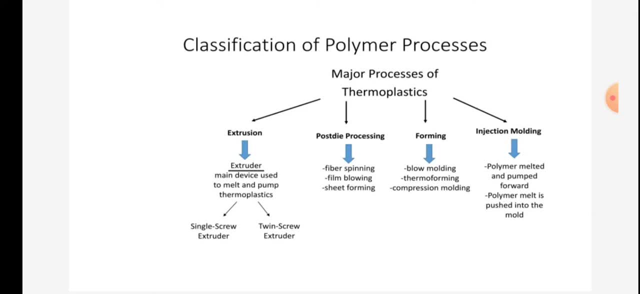 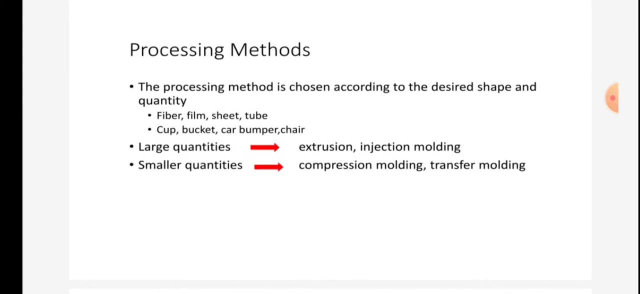 In this the processing method is given by polymer melted and الح场式 blending Process method is Groundlock´s method. according to desire, shape and quantity: Fiber, film, sheet and tube. A획: anonym Cup bucket, car bumper, chair, Large quantities, Extrusion injection訂верing. 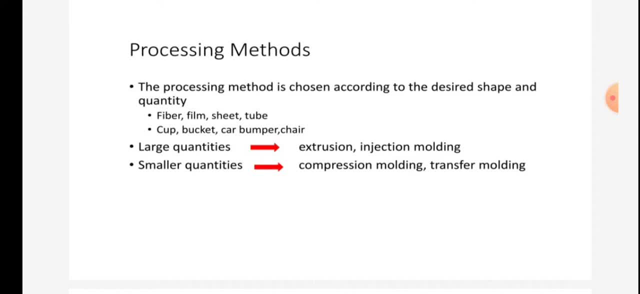 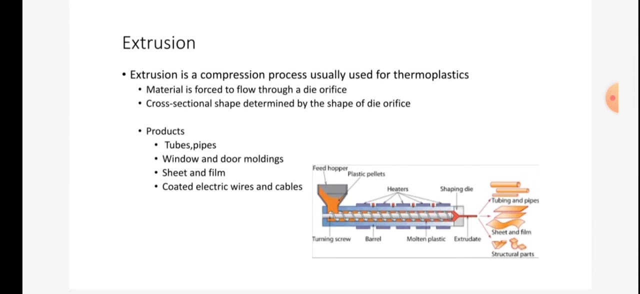 Injection molding. Large quantities of processing are used- extrusion and injection molding. Small quantities used compression molding and transfer molding. Extrusion: Extrusion is the compression process usually used for thermoplastics. Material is forced to flow through the die orifice. 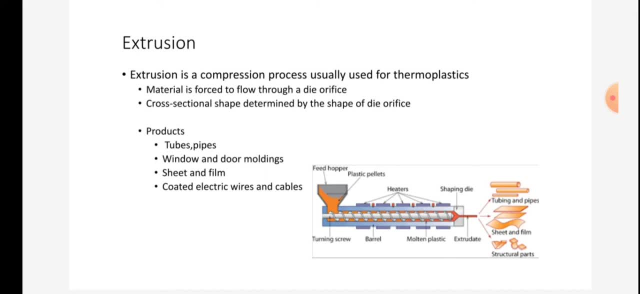 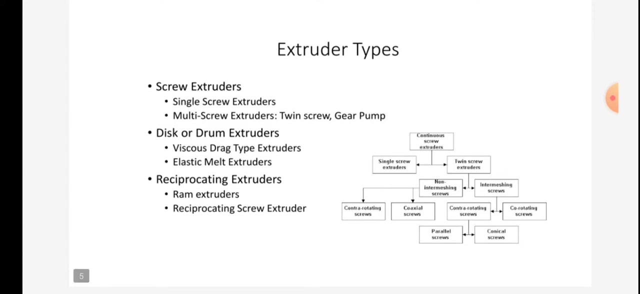 Cross-sectional shape determined by the shape of the die orifice Products: Tubes, Pipes, Window and door Moldings, Sheet and film Coated Electric wires, Cables. These are the manufacturers of extrusion Extruder types: Screw extruders. Screw extruders are classified as below: 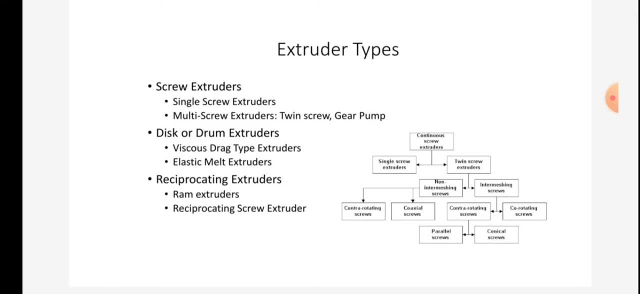 Single Screw extruders. Multiple screw extruders. Multiple screw extruders. Twin screw gear pump- Gear pump. This are drum extruders. Viscous drag type extruders. Elastic melt extruders. Reciprocating extruders are given as Classified as follows: 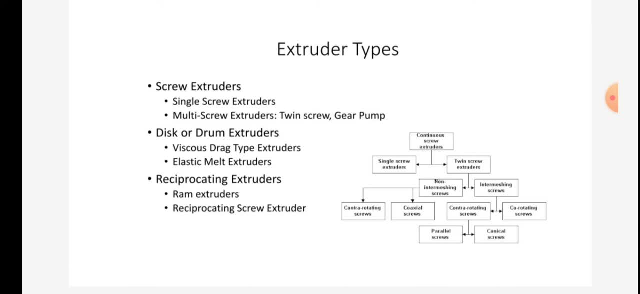 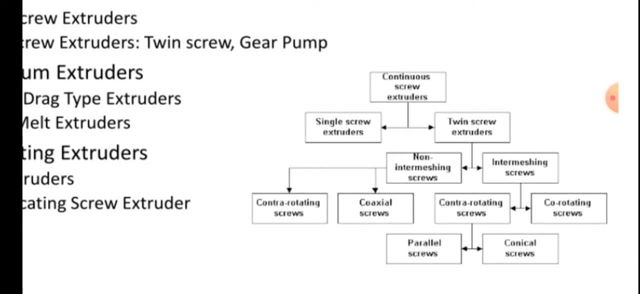 Ram extruders and reciprocating screw extruders. now we see continuous extruder. extruders are classified into two types: single screw extruders, twin screw extruders. now twin screw extruders are non-intermeshing screw screws and intermeshing. 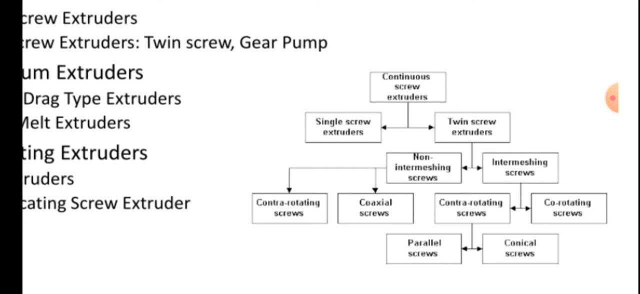 screws. in non-intermeshing screws, extra rotating, contra rotating screws, coaxial coaxial screws and in intermeshing screws, contra rotating screw, co-rotating screw and in contra rotating screws, parallel screws and conical screws. these are the classification of extruder types in 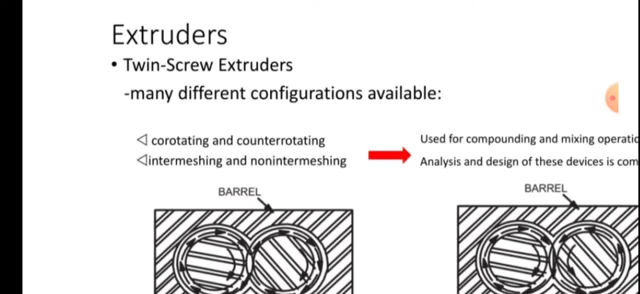 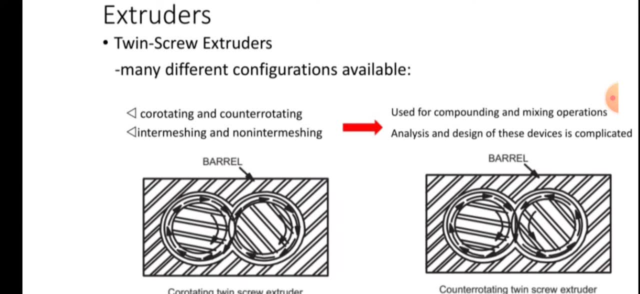 extruders: extruders- twin screw extruders- many different configurations available: co-rotating and contra rotating, co-rotating and contra rotating, then intermeshing and non-intermeshing in co-rotating and contra rotating used for compounding and mixing operations and intermeshing. and. 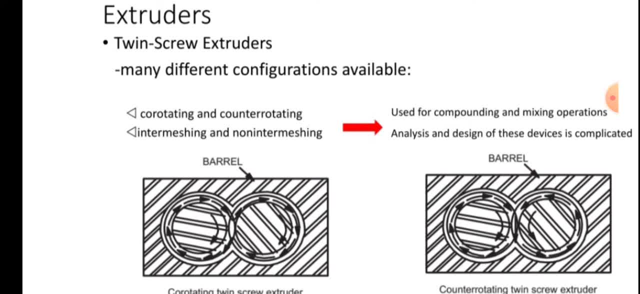 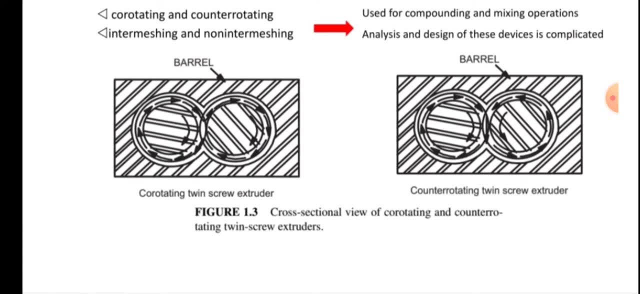 non-intermeshing are used for. analysis of and design of these devices is complete, complicated barrel is given. the figure shows the cross-sectional view of the co-rotating and counter-rotating twin screw extruders. it is shown in the figure of the co-rotating and non-intermeshing screw. 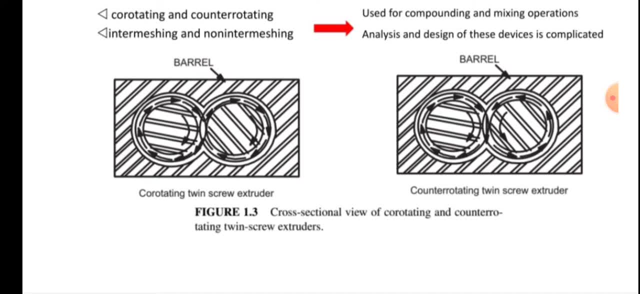 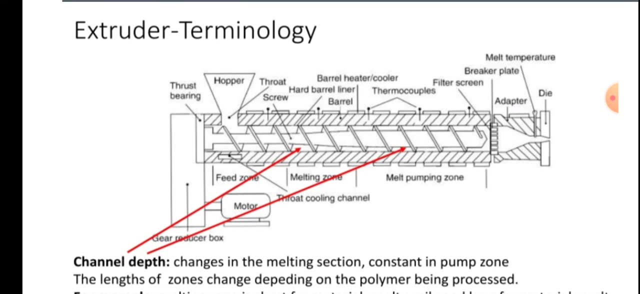 it is shown in the figure of barrel, and co-rotating twin screw extruders are shown in figure. again. barrel is given for counter-rotating 2nd screw extruders. extruder terminology. extruder terminology is given as below: thrust bearing is given in: 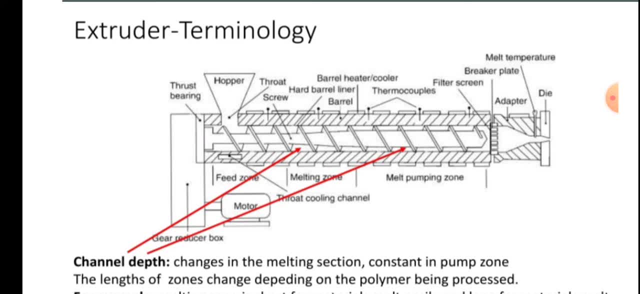 the figure hopper throat screw, modulate on this figure- can be used for any type of extruders: Hard Barrel Liner, Barrel Barrel Header, Heater, Barrel Heater or Cooler, Thermocouples, Filter, Screen Breaker, Plate, Melt Temperature, Die Adapter and then Feed Zone, Melting Zone Melt Pumping Zone, Throat Cooling Channel, Motor. 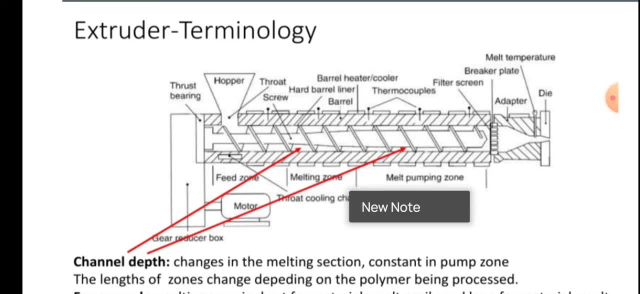 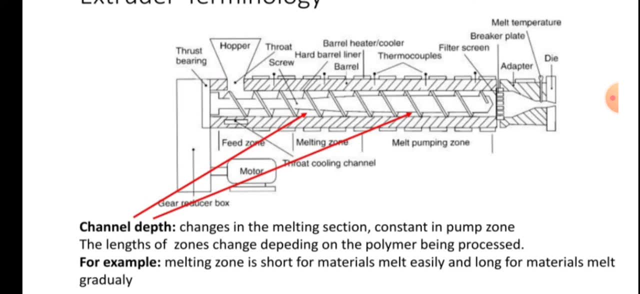 These are the parts of Terminology. Extra Terminology: Gear Reducers, Box Canal Depth. Changes in the Melting Section, Constant in Pump Zone. the Length of Zone Change depending on the Polymer being processed. For example, Melting Zone is short for 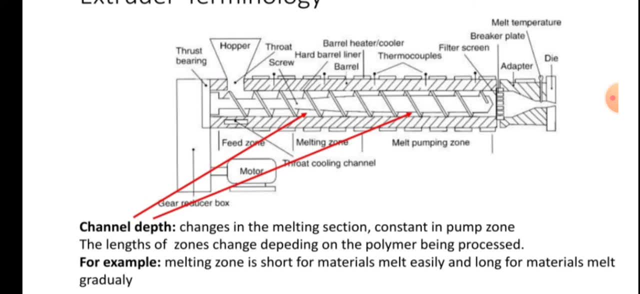 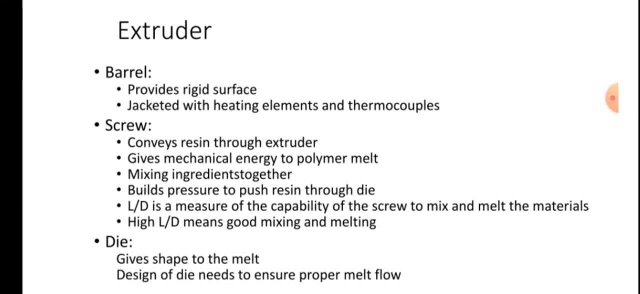 materials melt easily and long for. materials melt gradually. Now, Extruder Extruders are as defined as or classified as: and classified as follows: Barrel provides rigid surface jacketed with heating elements and thermocouples. Screw conveys resins through. extruder gives mechanical energy to polymer melt. 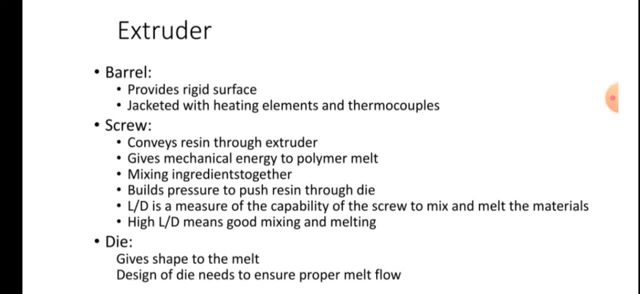 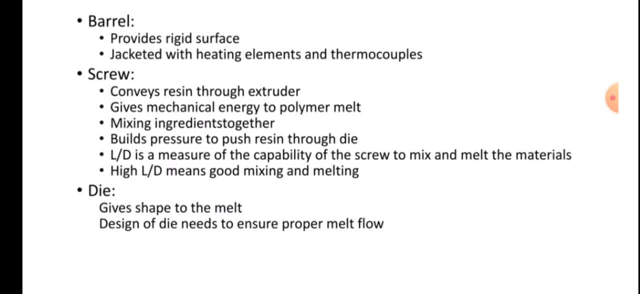 mixing ingredients together builds pressure to push resin through die linear L to D length to die and diameter is 0.5 mm. The diameter is 0.5 mm. The diameter is 0.5 mm. The diameter is 0.5 mm.